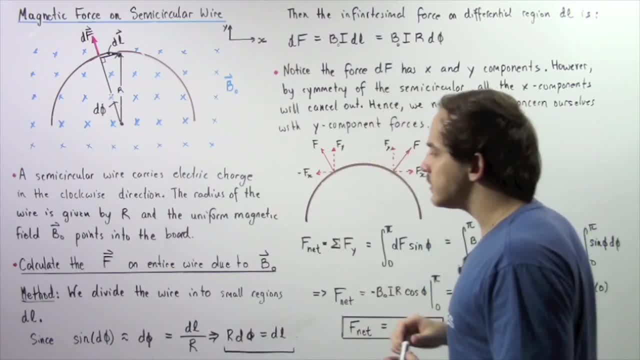 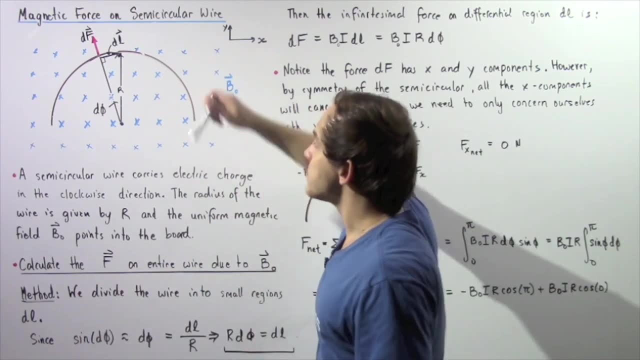 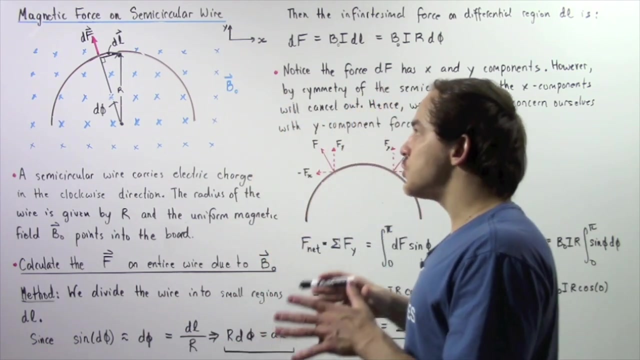 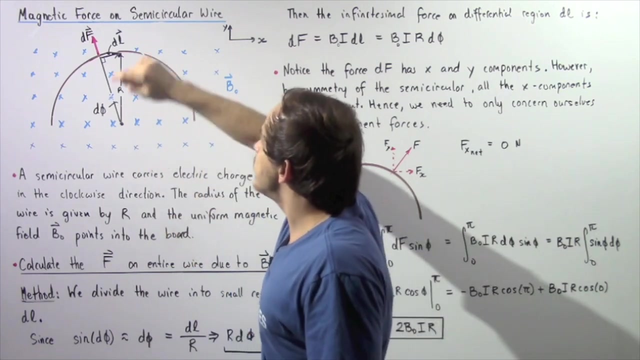 straight but because it's curved, we essentially have to divide the wire into very short regions given by the differential DL. So this quantity, DL, is an infinitely small quantity. So we essentially want to ask ourselves what exactly is the infinitely small force given by DF that is acting? 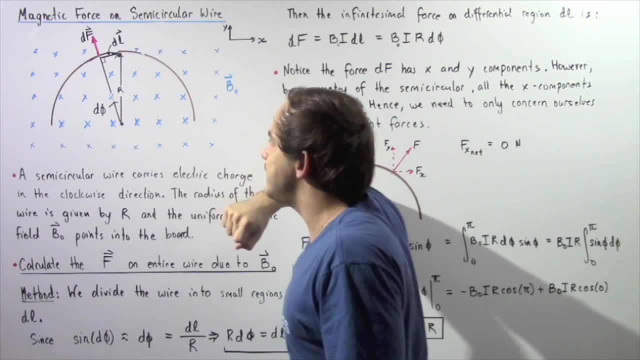 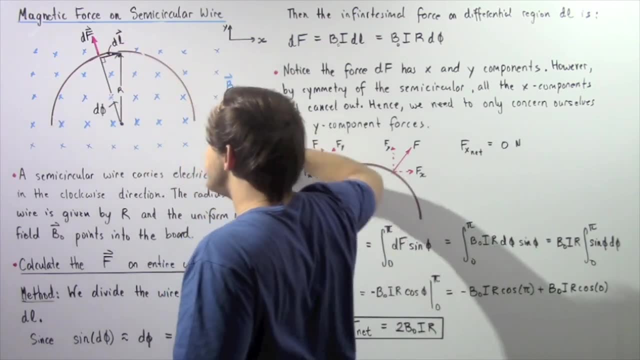 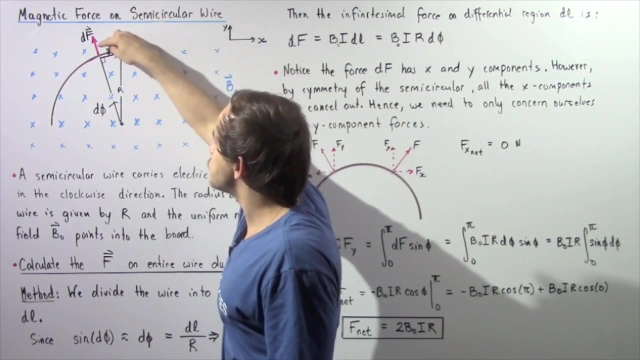 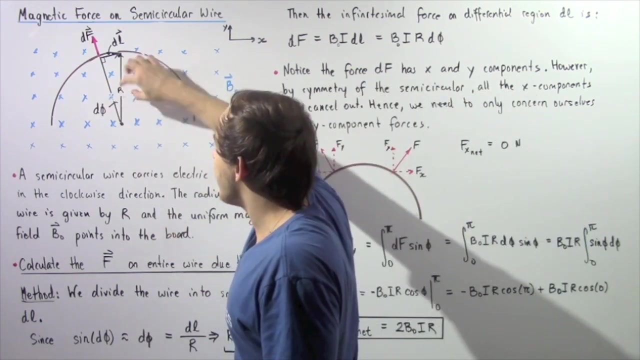 on the following infinitely small region given by DL. So if we calculate what that force is and then we integrate over this entire region, that will give us our net force. So before we go into that, let's take this differential DL and let's try to represent that differential DL in terms of the angle D5 and the radius of our 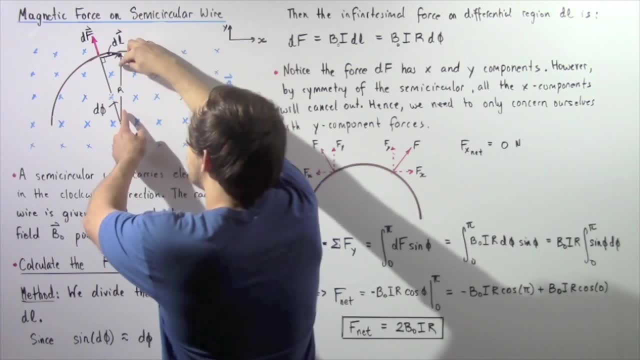 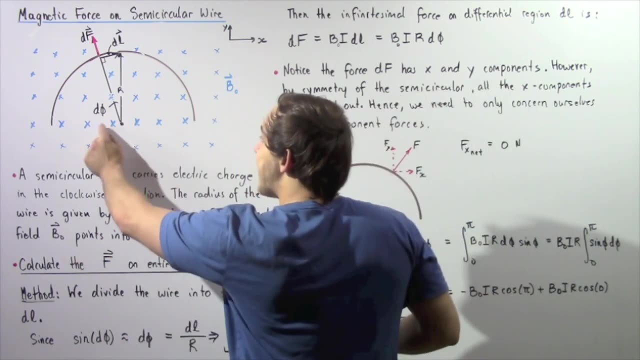 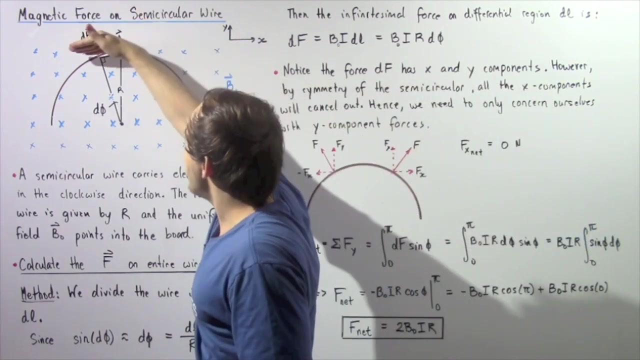 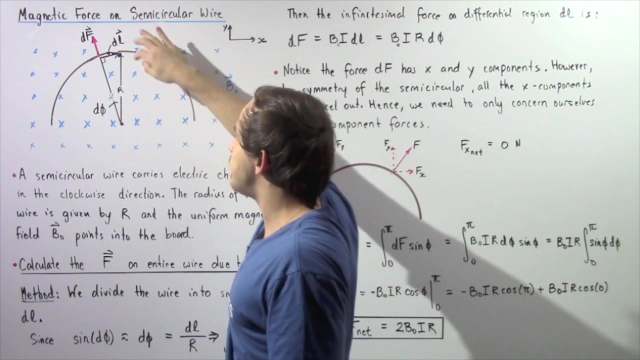 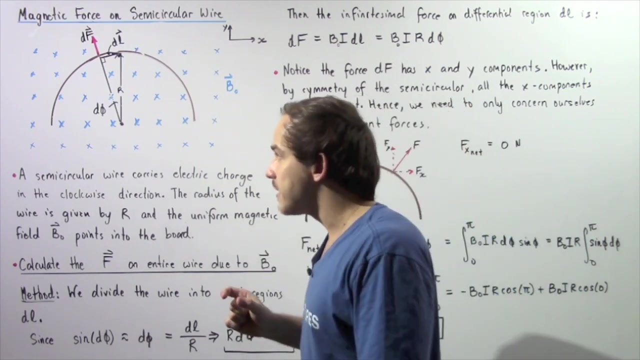 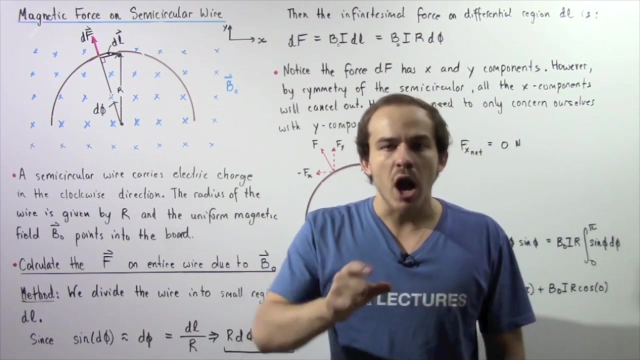 semicircle. So we essentially draw the following right triangle and we use our sine trigonometric function, So sine of this angle given by D5, our infinitely small quantity is acting on the which is equal to the angle D5, which I get the 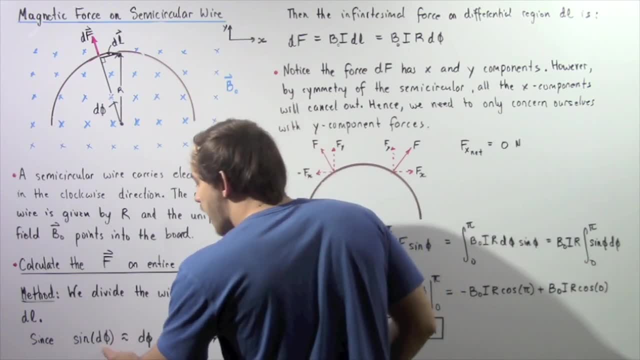 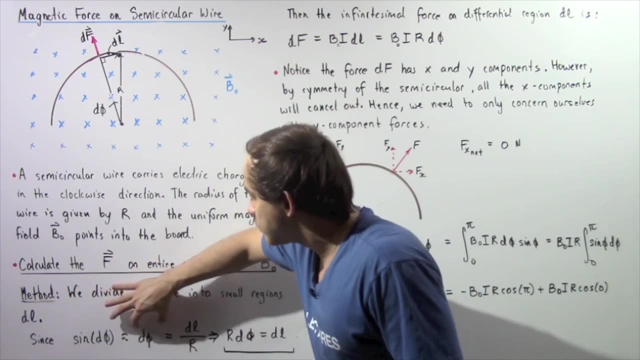 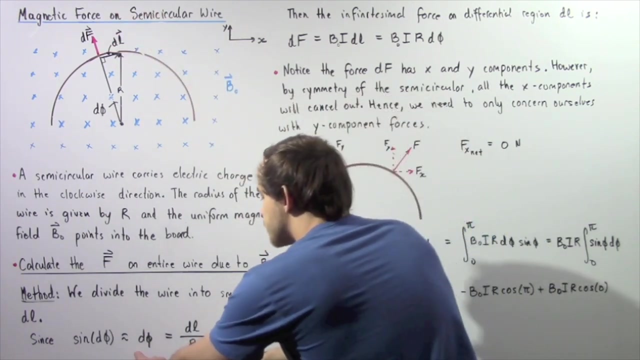 ugen, ironically enough, 2-th times its length of theецicections. So this part, 2-th time, this marginal of the infinitely small angle d phi is approximately equal to the angle d phi And that implies, because this is equal to this, d phi is equal to our dl divided by r. So we take this equation. 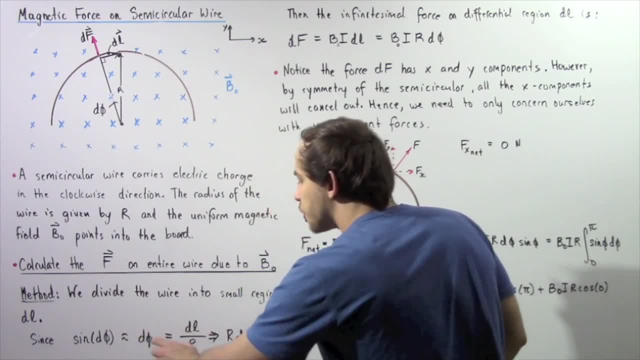 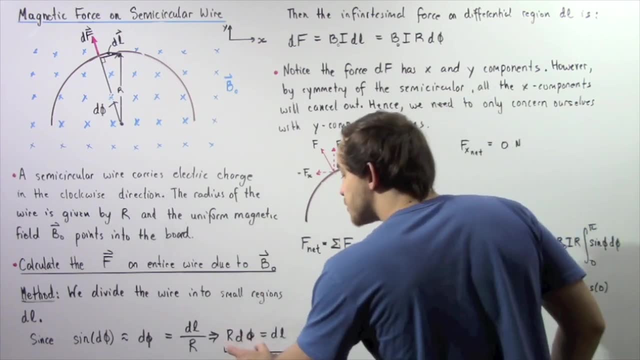 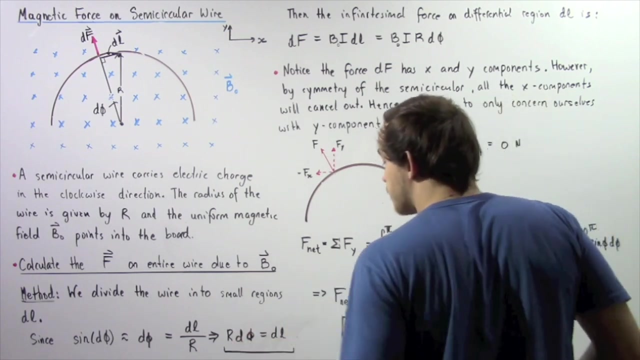 and we represent this equation, dl, in terms of d phi and r. So we see that dl is equal to r, the radius multiplied by this infinitely small angle given by d phi. So this relationship will become important in just a moment. So now we want to calculate what this infinitely? 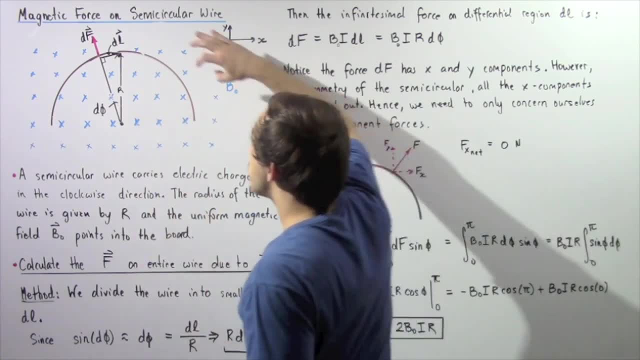 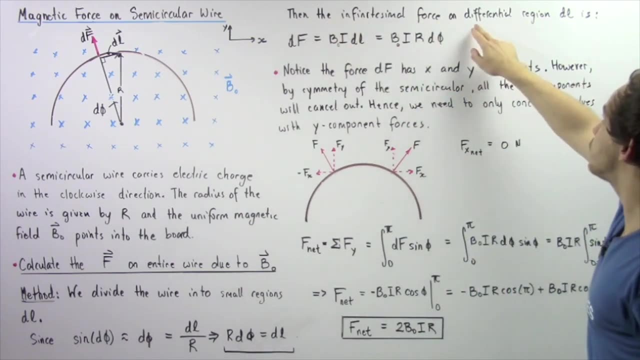 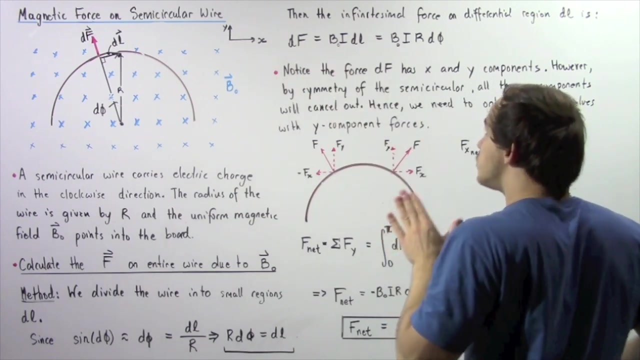 small force is df, that is acting over this infinitely small region given by dl. So the infinitely small force on our differential region, dl, is equal to the following equation, equation which we spoke about in a previous lecture. So we said the force Df on this infinitely small region, DL, is equal to the product of: 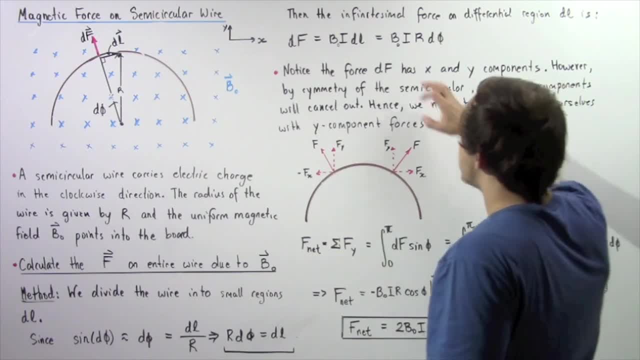 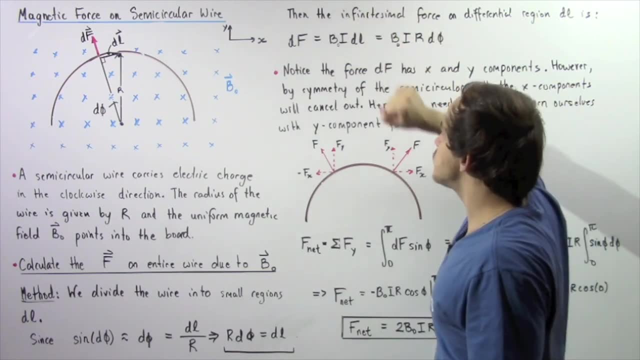 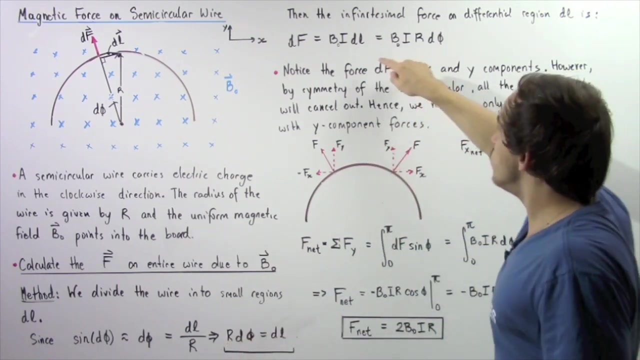 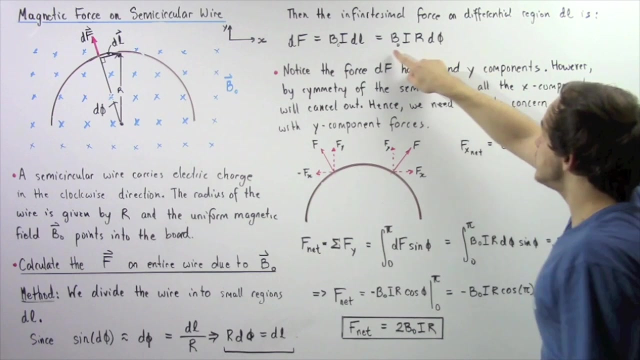 our constant magnetic field, B0, multiplied by the electric current I that flows through our wire, multiplied by our infinitely small region, given by DL. Now, because DL is equal to R multiplied by D phi, we can replace DL with R multiplied by D phi. So our infinitely small force, Df, is equal to the following product of these four quantities: 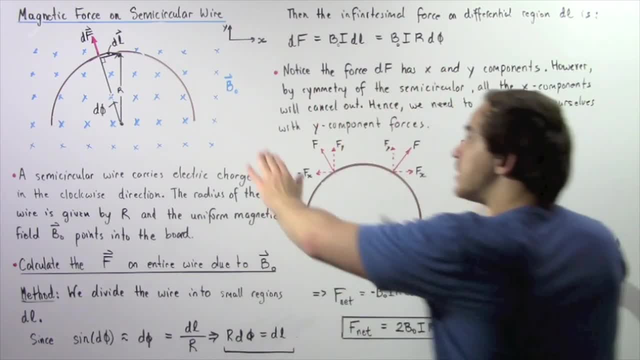 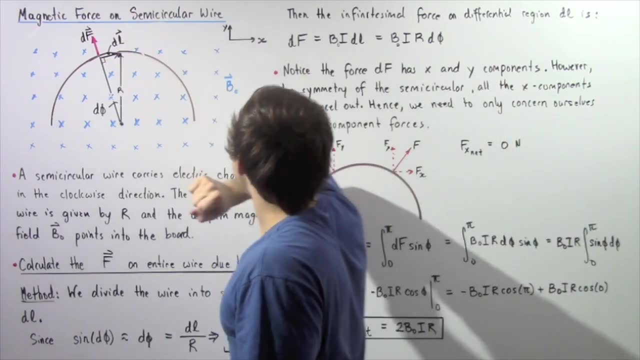 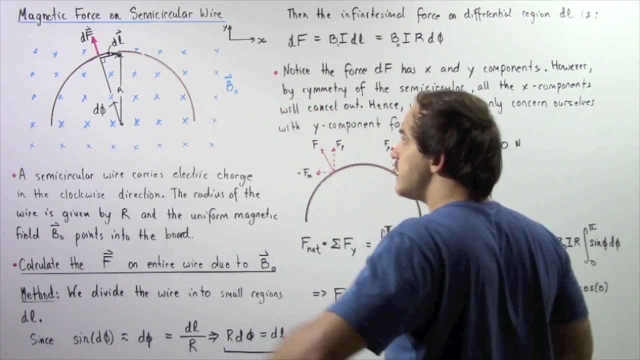 Now let's notice the following important point about the symmetry of our semicircle. So notice, if we examine this force and we choose our x-axis to lie along this And the y-axis to lie along this direction, we see that this force will actually have. 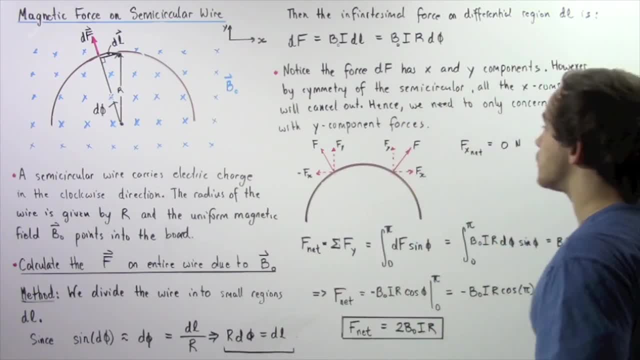 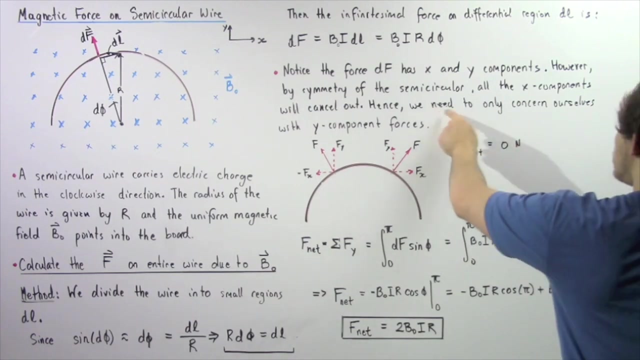 a y-component force as well as an x-component force. So notice: the force Df has x and y components. However, by the symmetry of the semicircle, all the x components will cancel out. Therefore, we need to only concern ourselves with the y-component forces. 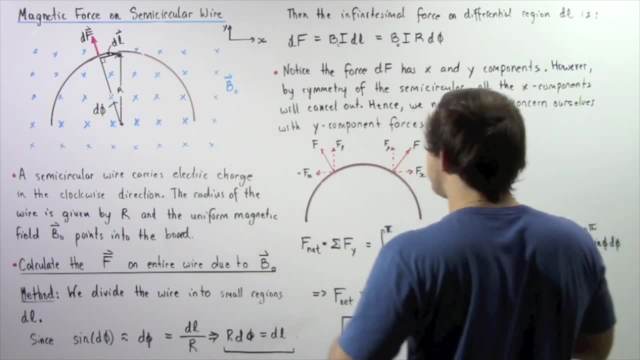 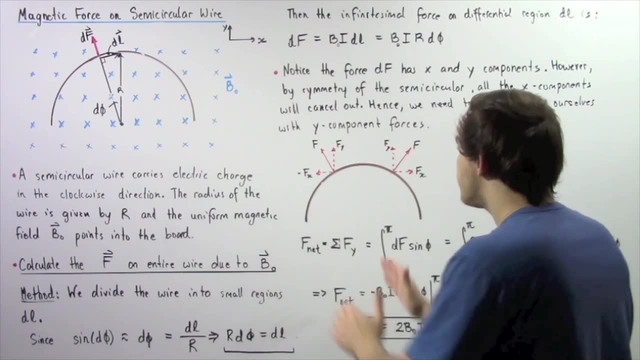 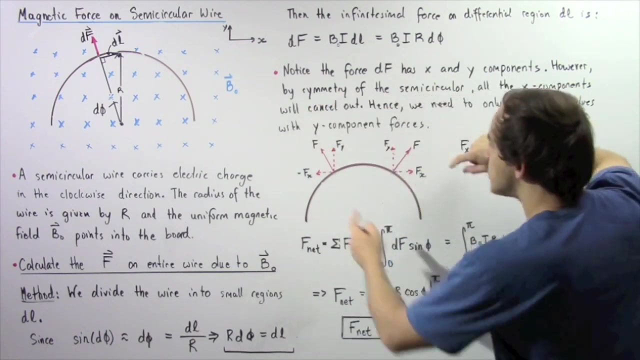 So let's see exactly what that means by looking at the following diagram. So notice: this semicircle is symmetrical. If we cut it in half, this region will be exactly the same as this region. So let's take this force and let's look at the force across. 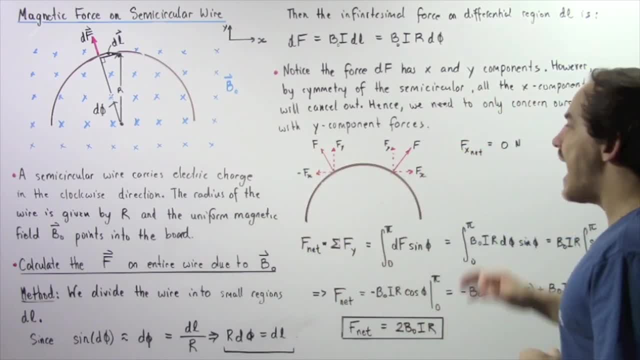 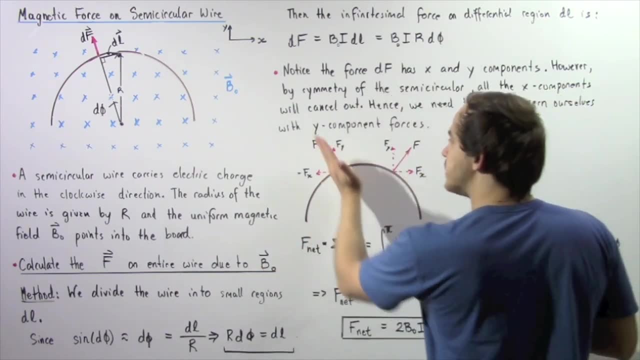 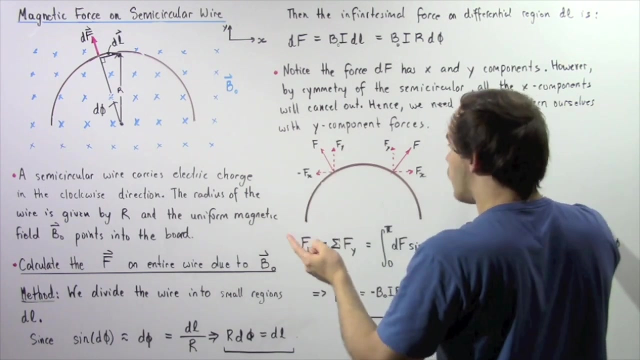 So these forces will each have an x-component and a y-component force. So we essentially use the right hand rule And we see that the force At this region points this way. The force at this region points this way. Now these two forces will have an x-component. 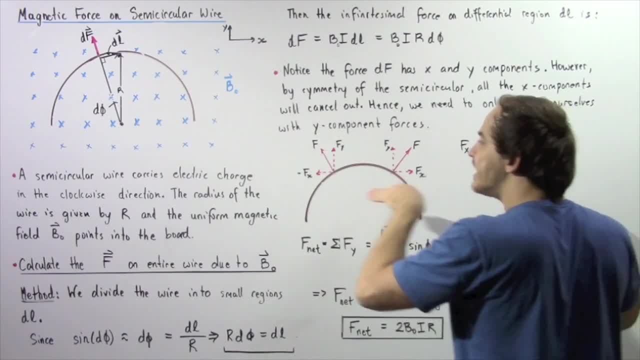 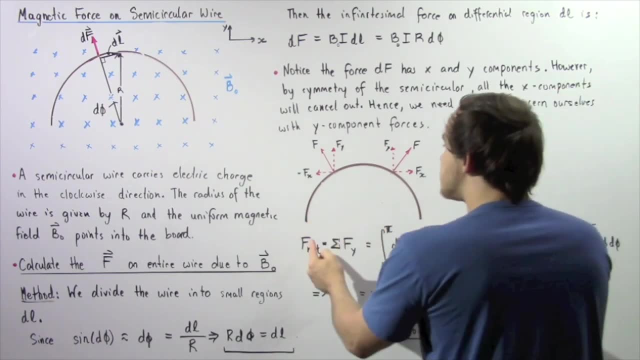 One will point in this direction, The other force will point in the opposite direction. So if we take the sum of these forces, they will cancel out. In fact, if we sum up all the forces acting along the x-axis, that will give us zero, as. 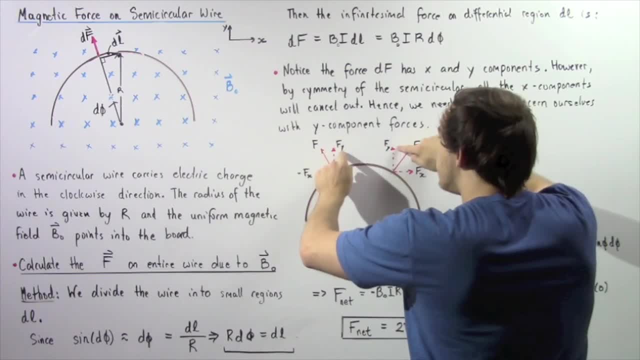 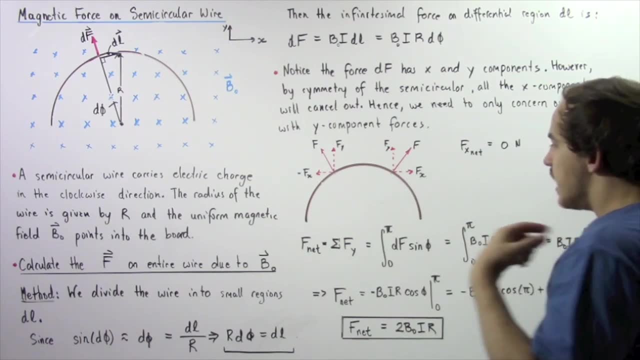 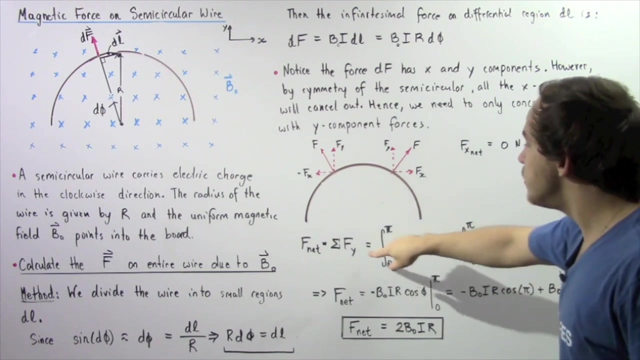 a result of this symmetry, However, The y-component forces Point in the same direction, So that means they will not equal to zero. So the net force acting on this entire region as a result of our constant magnetic field is equal to the sum of all the forces acting along our y-direction. 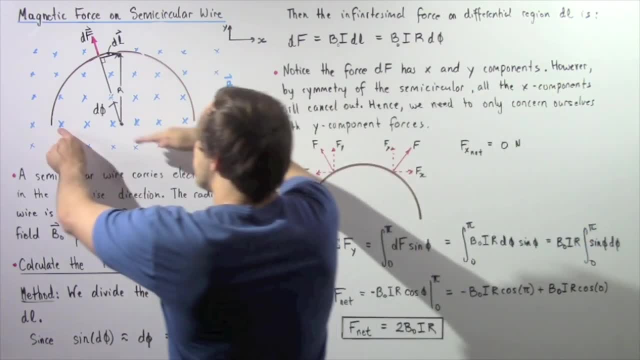 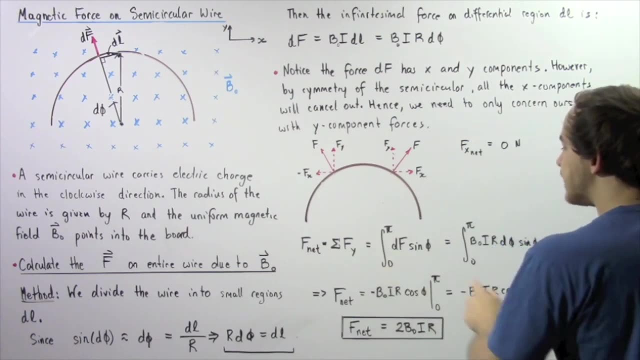 And this is equal to the integral from angle of zero to angle of pi, which is equal to 180 degrees. So that is equal to zero. So we are still right at the point in time. Now we can see that the force at this region was equal to the angle of pi. 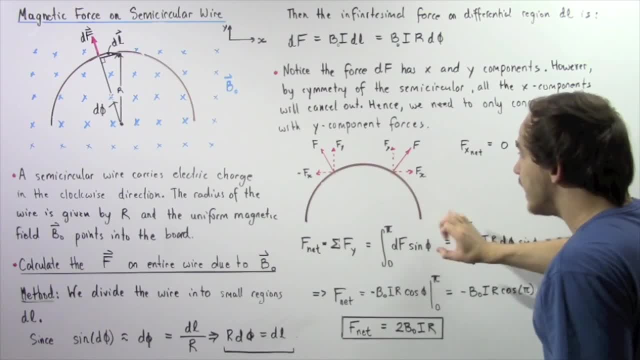 Now, this is equal to the sum of all the forces acting along the x-axis, and this is equal to zero. So what is the sign of the angle of pi? It is equal to phi, And so in this case we have the line f multiplied by the angle of pi. 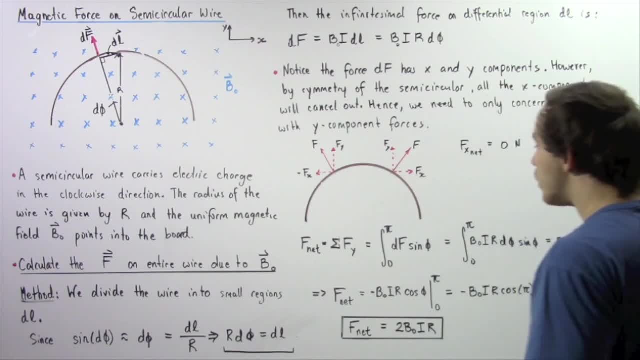 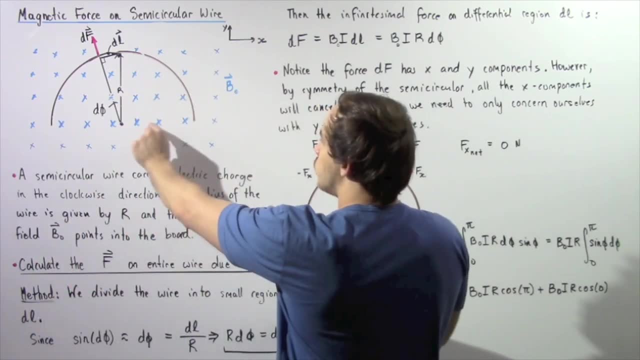 Now df is the sine of the angle of pi. Now df is simply our y-component force. So once again we are integrating from an angle of zero. We are assuming this is our angle zero and this is our angle 180.. So zero to 180, because we want to use radians. 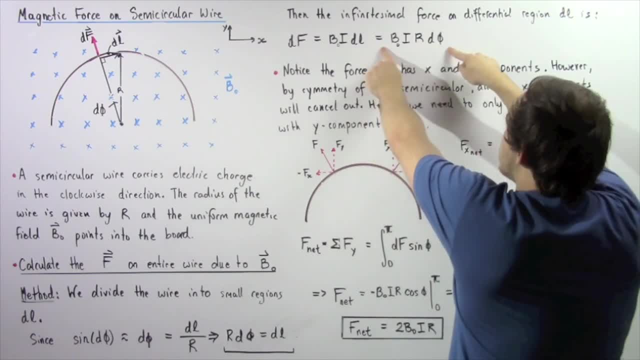 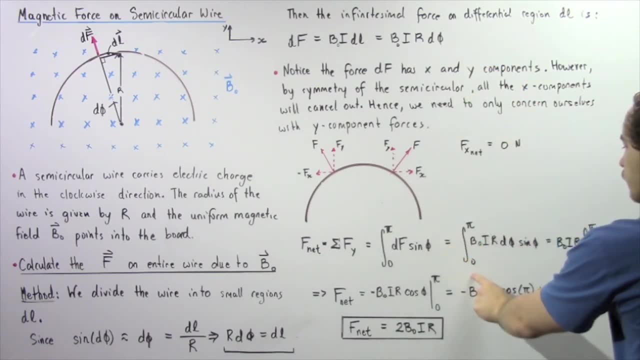 So now we know that df is equal to the following product, So we know that we are going to integrate from this angle to this angle So we can replace df with this entire product. So this is equal to the integral from 0 to pi of b0 multiplied by r. 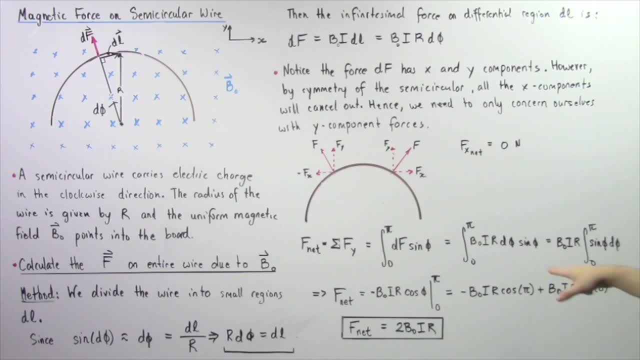 multiplied by i, multiplied by d phi, multiplied by sine of phi. Now these three quantities are all constants, so we can bring them outside of our integral and we get the following result: Now, if we actually integrate, this becomes negative and sine phi becomes cosine phi. 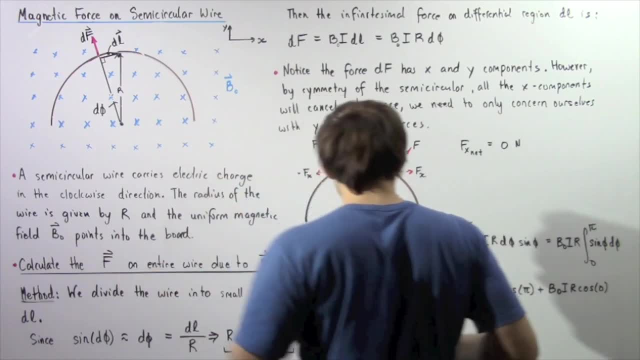 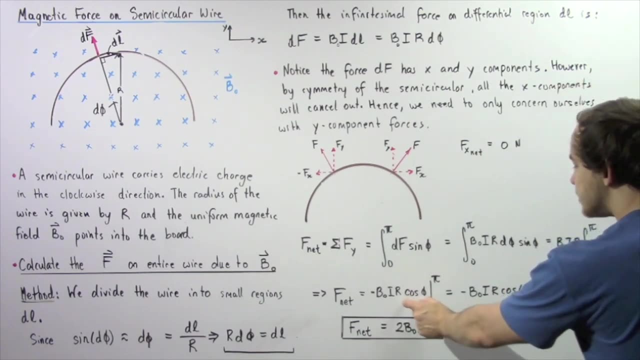 So we see that the net force acting on this entire region is equal to negative magnetic field multiplied by current, multiplied by radius, multiplied by sine of phi, from 0 to pi. So if we evaluate the integral, we get the following result: Now, cosine pi is equal to negative 1..